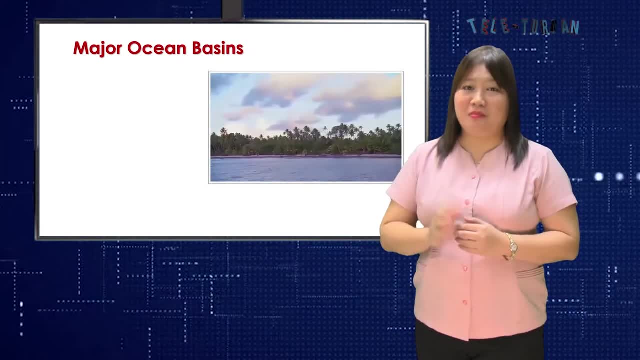 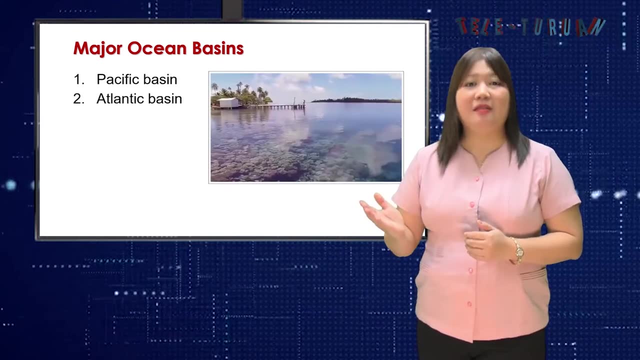 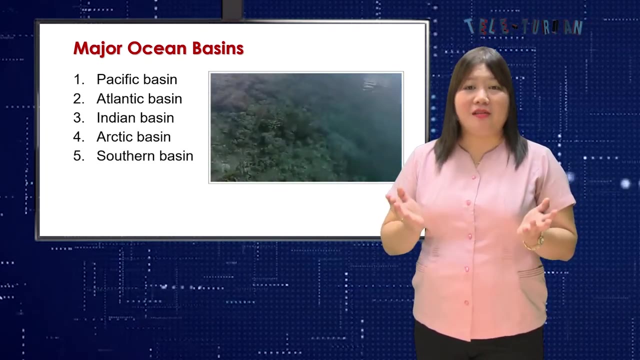 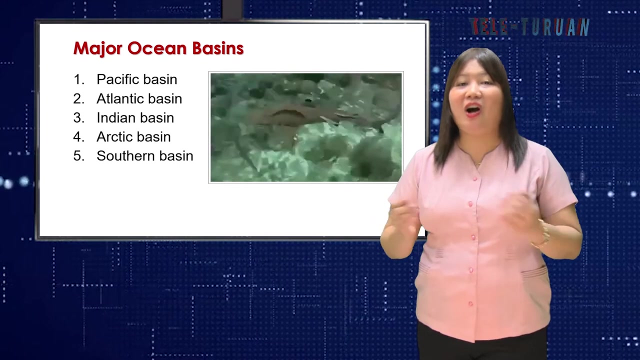 There are five major ocean basins coordinating with the major oceans of the world: The Pacific Basin, the Atlantic Basin, the Indian Basin, the Arctic Basin and the Southern Basin. Many smaller basins are often considered oceanic basins, such as the North Alethean Basin between the Pacific and Arctic Oceans. 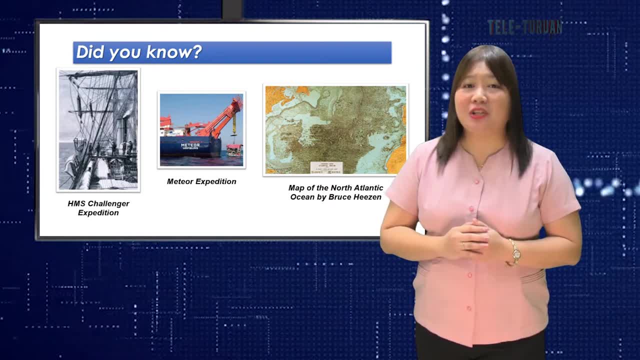 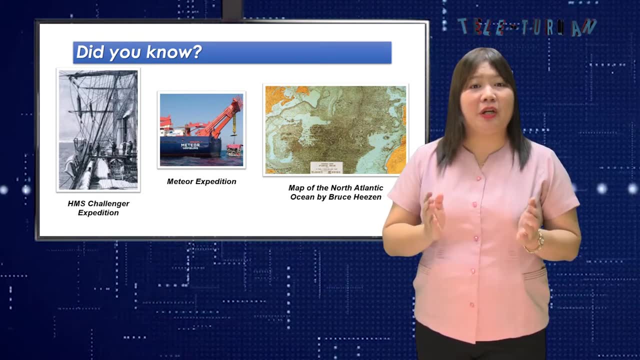 Did you know? The HMS Challenger is a major ocean basin. The HMS Challenger is a major ocean basin. The HMS Challenger is a major ocean basin. The HMS Challenger Expedition made the first attempt to measure the water depth with winches and cables, and the Meteor Expedition was the first to measure water depth with acoustic methods, using echo sounding. 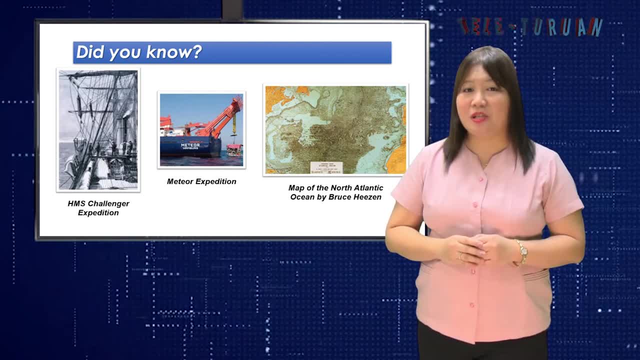 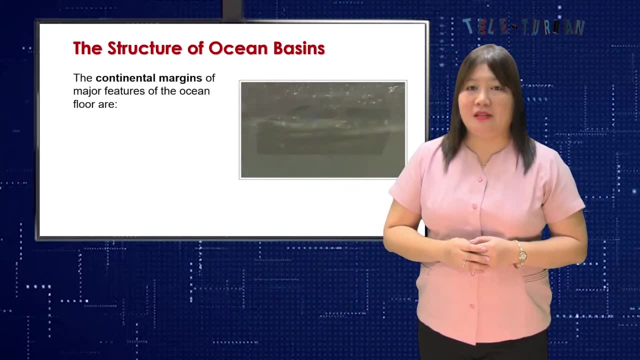 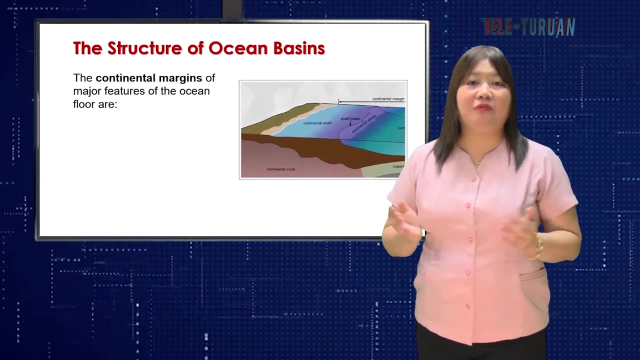 On the other hand, the first public map of the North Atlantic Ocean Basin was published by Bruce Heason in 1959.. The structure of ocean basins involves measuring the size and shape of the Earth's ocean basins. The continental margins of major features of the ocean floor are: 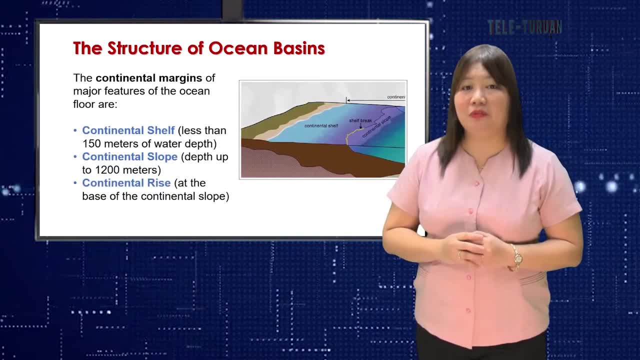 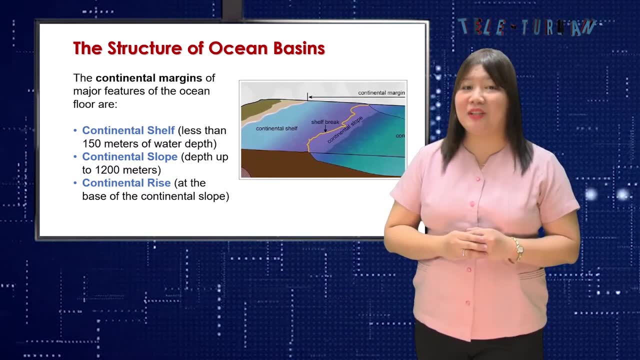 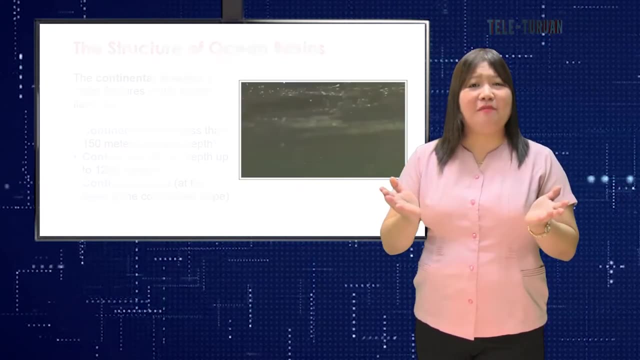 Continental Shelf with less than 150 meters of water depth, Continental Slope or Steep Ramp to a Depth up to 1,200 meters, and Continental Rise is found at the base of the Continental Slope. Those types of margins may be Passive. whose shelf with hundreds of kilometers wide? 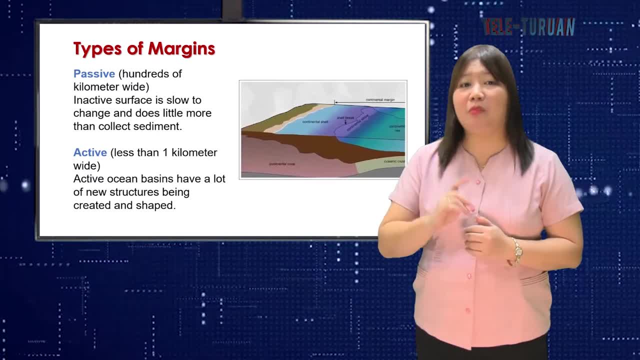 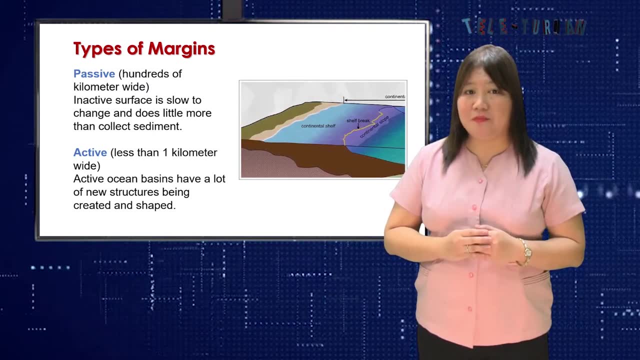 or Active, whose shelf may be less than 1,000 meters wide, and Passive, whose shelf with hundreds of kilometers wide, or Active, whose shelf may be less than 1,000 meters wide. Ocean basins can be either Active, with a lot of new structures being created and shaped. 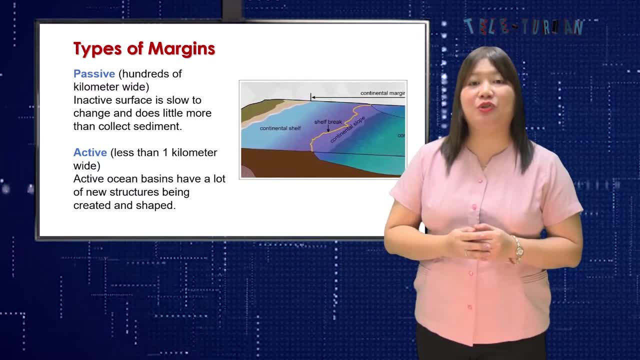 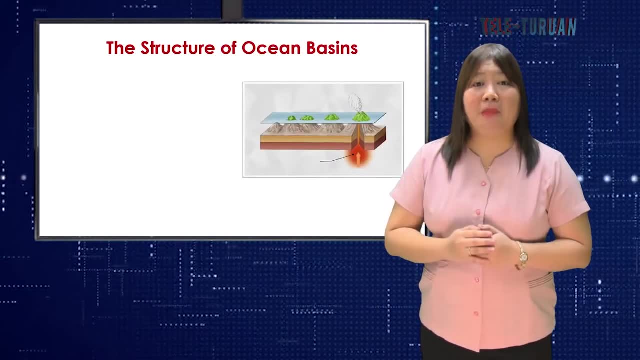 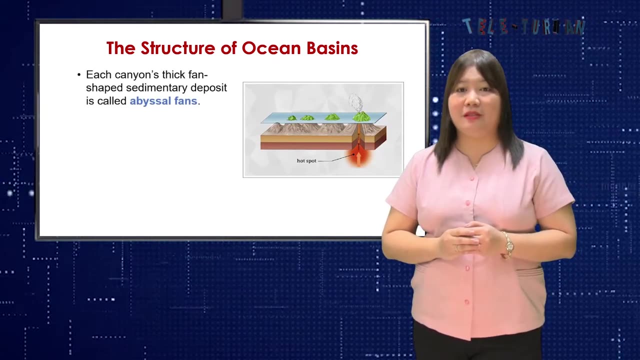 or they can be Inactive where their surface is slow to change and thus little more than collects sediment. All of those slopes are capped by submarine or V-shaped canyons. Each canyon's thick, fan-shaped sedimentary deposit is called an abyssal fan. 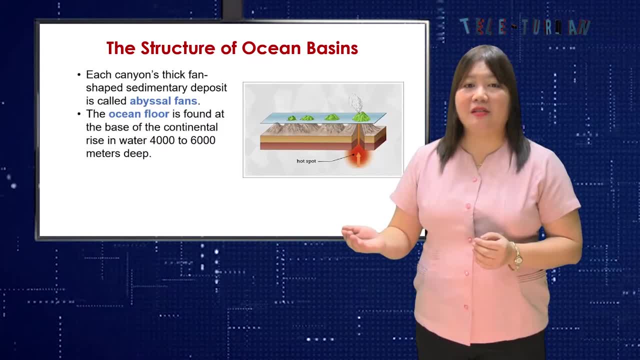 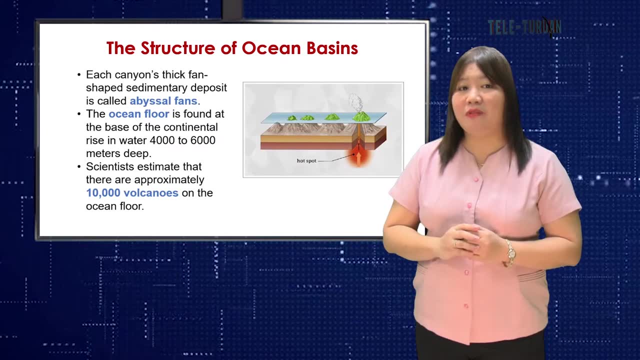 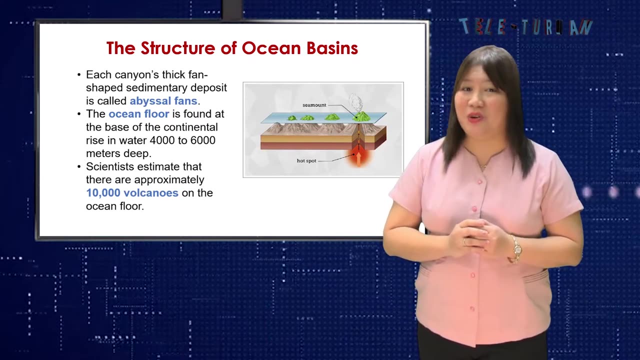 The ocean floor is found at the base of the Continental Slope. This is at an area with a continental rise in water 4,000 to 6,000 meters deep. Numerous volcanoes populate the floor of the ocean basins. Scientists estimate that there are approximately 10,000 volcanoes on the ocean floor. 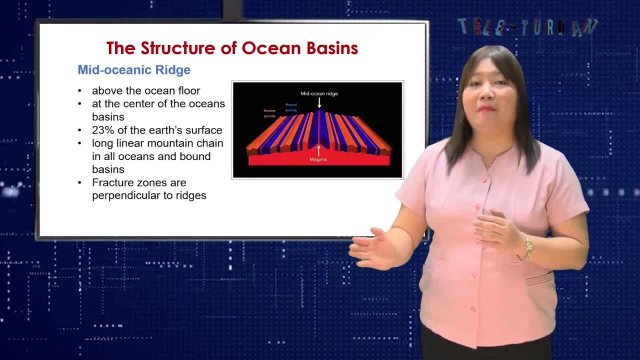 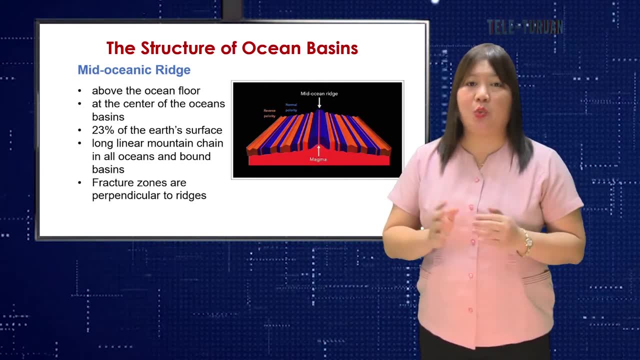 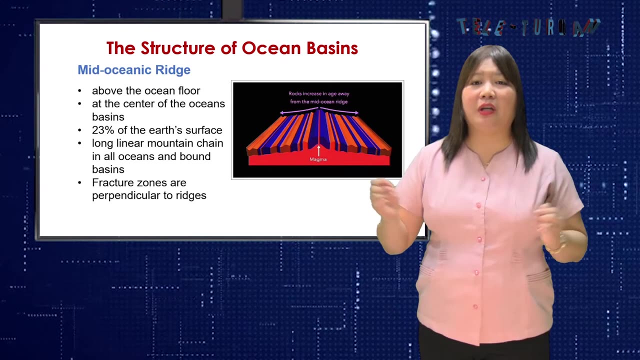 Mid-ocean ridge is normally found rising above the ocean floor at the center of the ocean basin. The mid-oceanic ridge constitutes 20% of the earth's surface. Mid-ocean ridges are long leader mountain chains which occur in all oceans and downed basins. 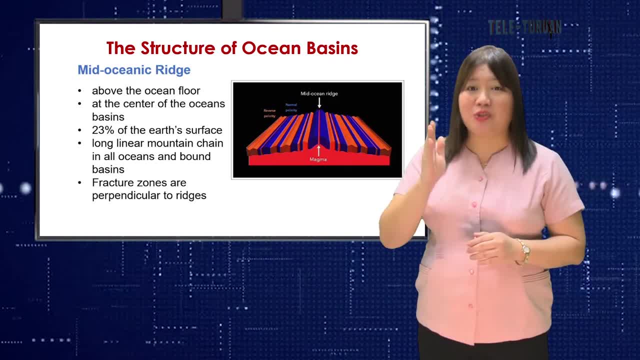 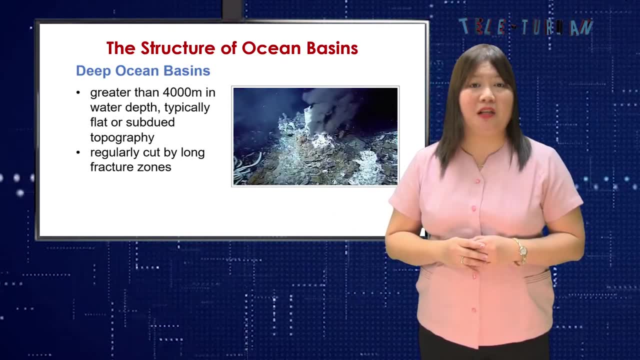 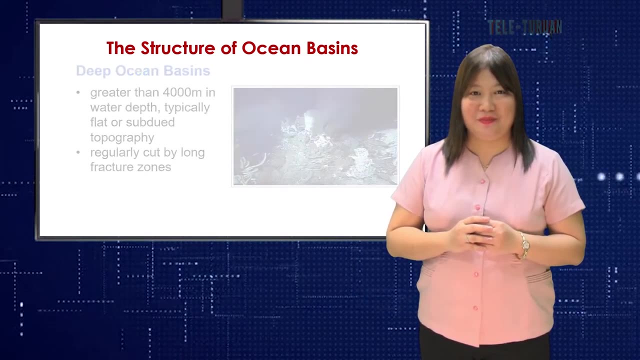 On the other hand, fracture zones are perpendicular to ridges. Deep ocean basins greater than 4,000 meters in water depth are typically flat or subdued topography and regularly capped by long fracture zones. Ocean trenches are long, narrow, steep-sided depressions found on the ocean floor. 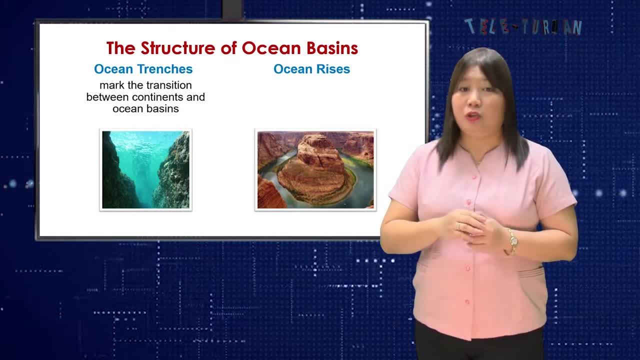 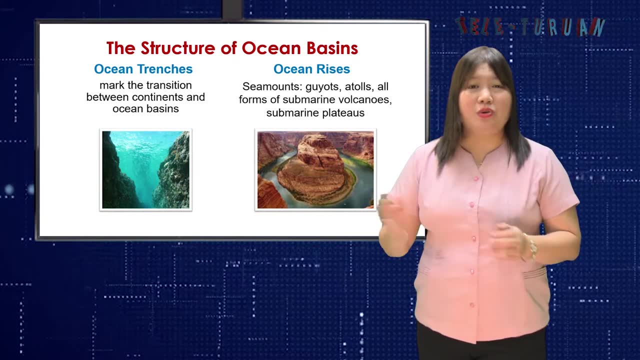 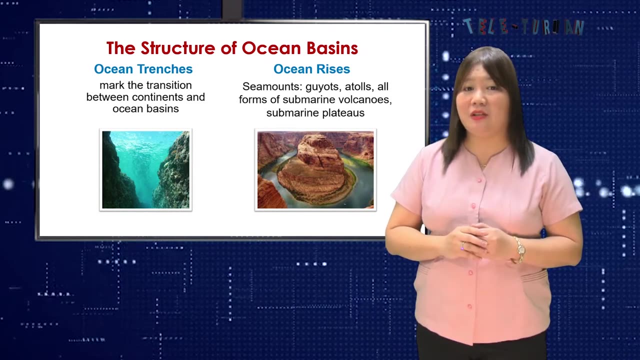 that contain the greatest depths in the ocean. They mark the transition between continents and ocean basins, especially in the Pacific basin. Ocean trices include seamounts such as geos atolls and all forms of submarine volcanoes and submarine plateaus. 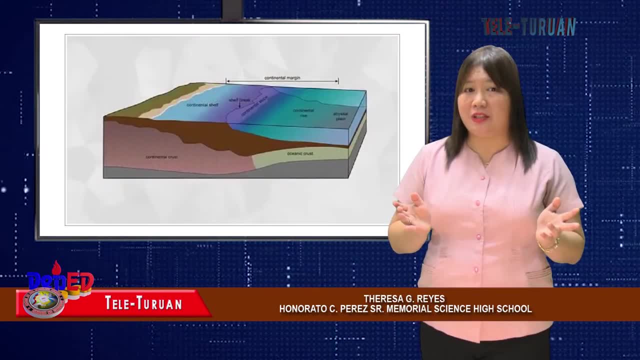 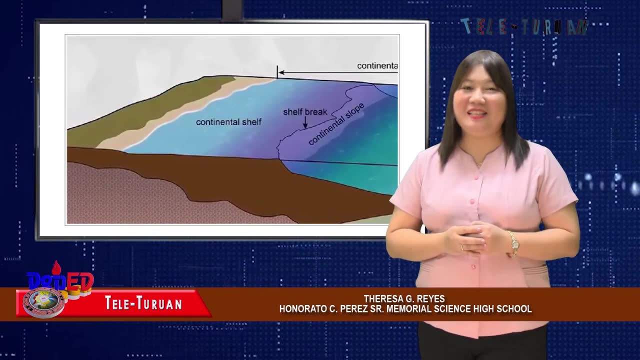 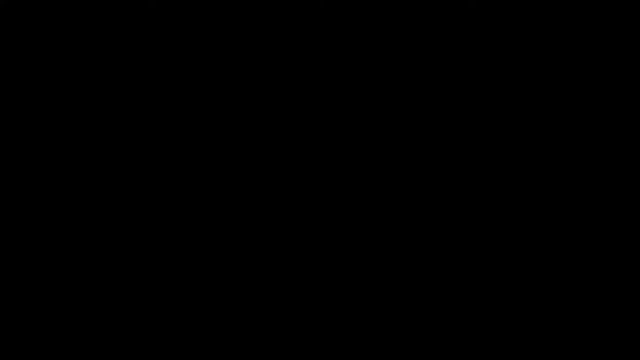 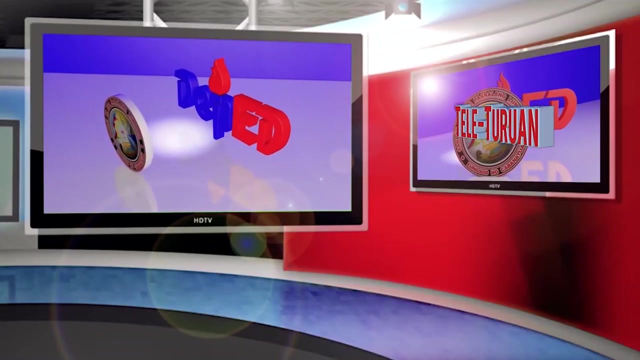 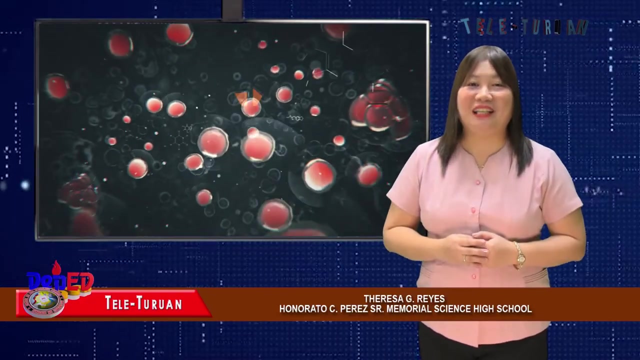 Now you know that ocean basins are the largest depressions on earth. I'll tell you more as we continue on the evolution of ocean basins when we come back after the break. Stay tuned. Welcome back here at Deped Hour. Teleturuan: Knowing the structure or formation of ocean. 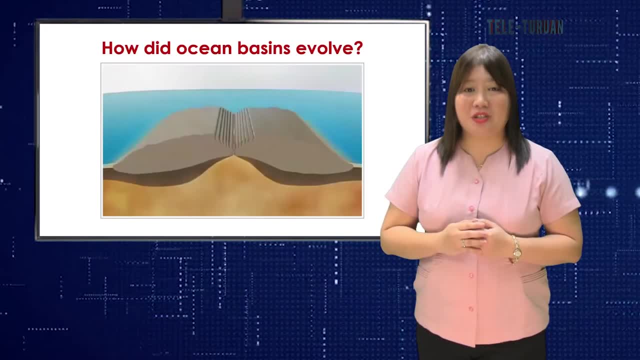 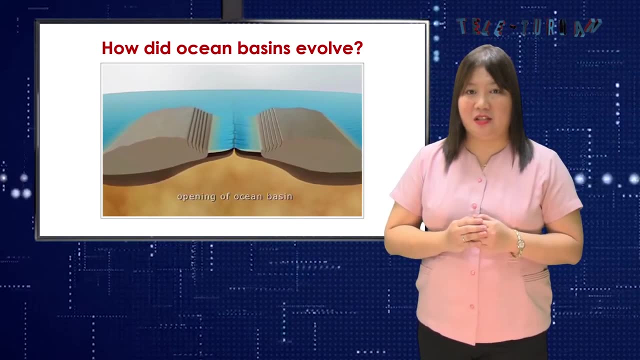 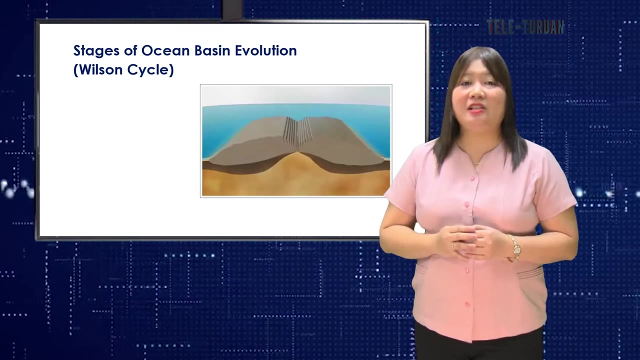 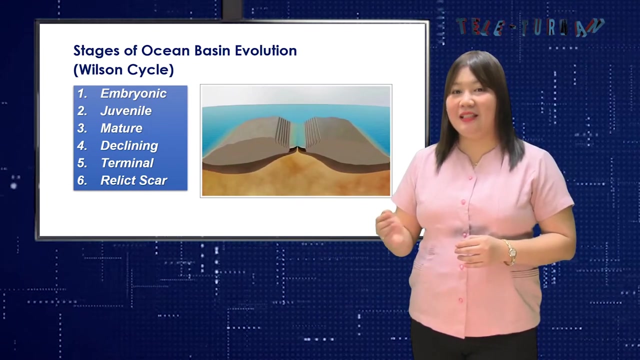 basins. next question is: how did ocean basins evolve? Different ocean basins are geomorphologically distinct based on their stage of geological evolution. according to the Wilson Cycle, The stages of ocean basin evolution include embryonic, juvenile, mature, declining, terminal and relict scar. Stage 1 is embryonic. Continental rifting plays a key role in the formation of ocean basins. Age of ocean basins are important for the development of ocean basins. There are many different stages of geomorphological evolution. The first is the stage where ocean basins 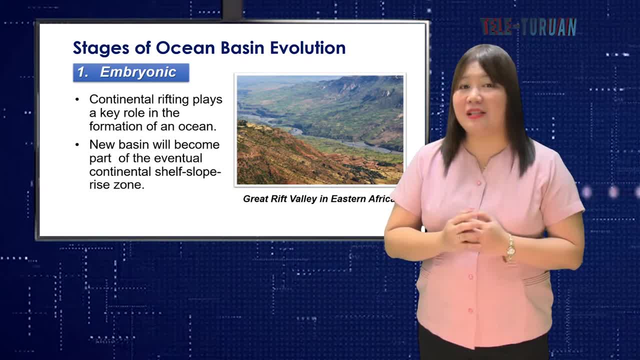 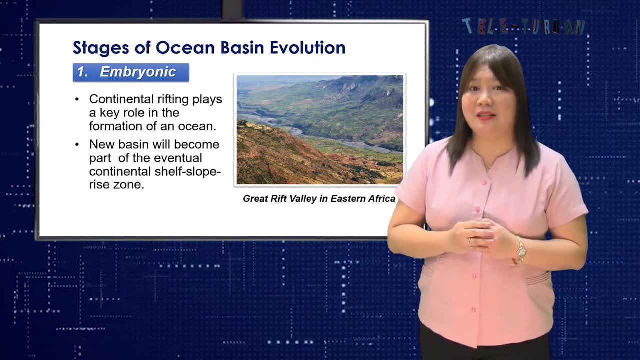 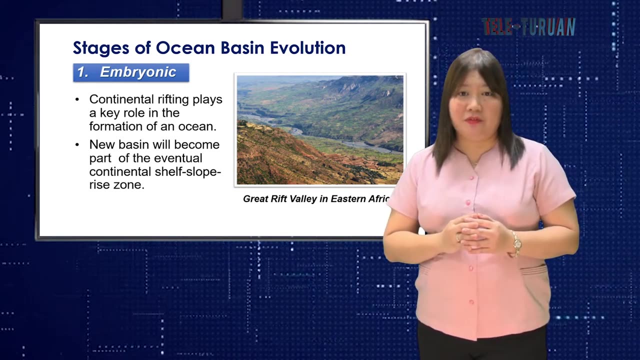 formation of an ocean Rift valley forms as continent begins to split. When separation does occur, sediments from the adjacent continents soon begin to build out into the new basin and will become part of the eventual continental shelf slope rise zone. An example is a great 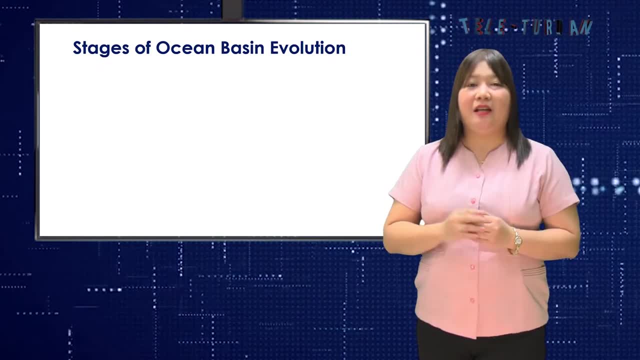 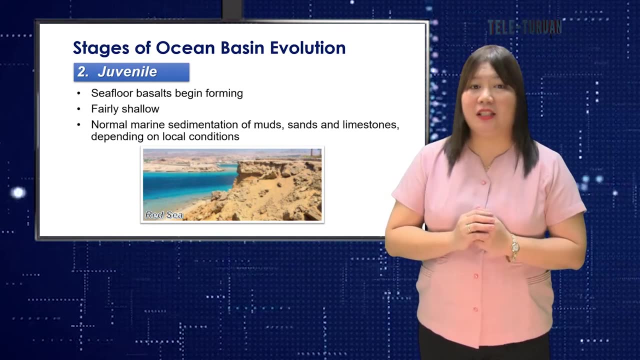 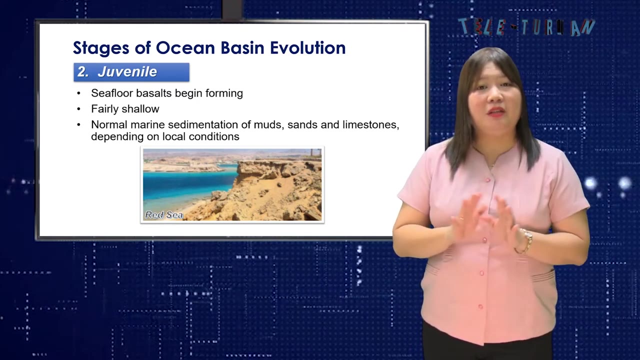 rift valley in eastern Africa. Stage 2 is described as juvenile Seafloor. basalts begin forming as continental sections diverge. Initially, the Yangmarine basin is fairly shallow. If repeated influxes of seawater become wholly or partly evaporated, salt deposits. 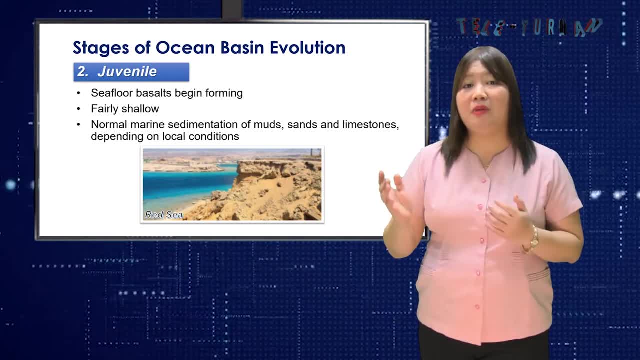 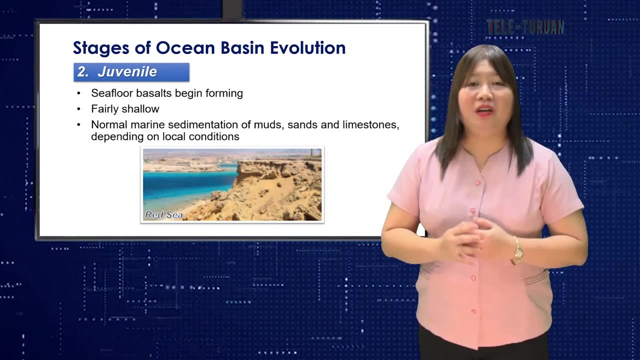 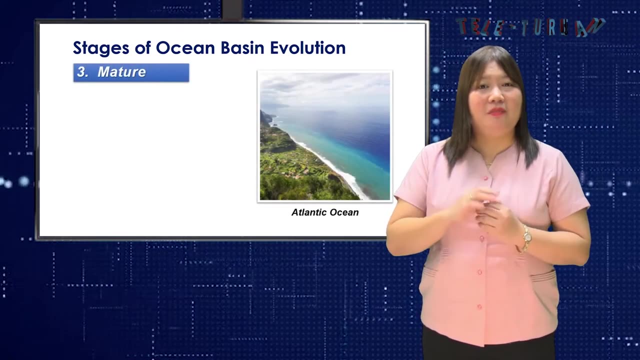 will accumulate. Otherwise, there will be normal marine sedimentation of muds, sand and limestones, depending on local conditions. One of the clearest examples of a Yang Ocean basin is the Red Sea. In stage 3, mature ocean basin becomes broad. 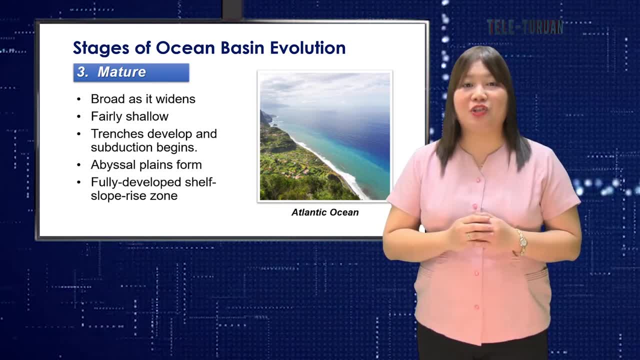 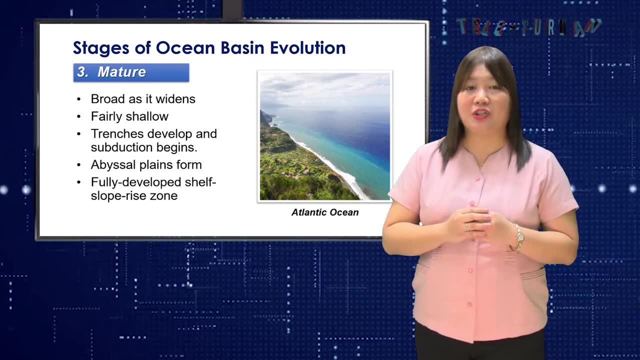 as it widens, Trenches develop and subduction begins. The ocean floor between the spreading axis and the continent subsides. by thermal contraction of the underlying lithosphere, Abyssal plains form and the continent subsides. The ocean floor is the first place where seawater 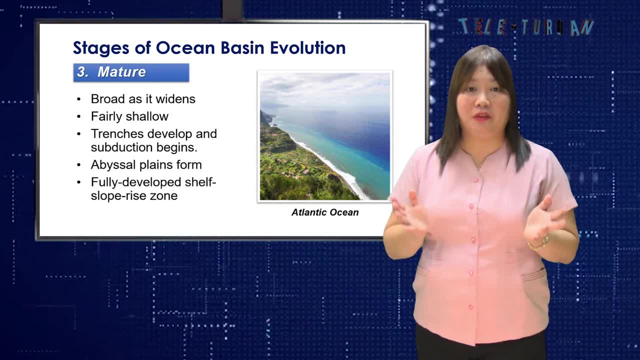 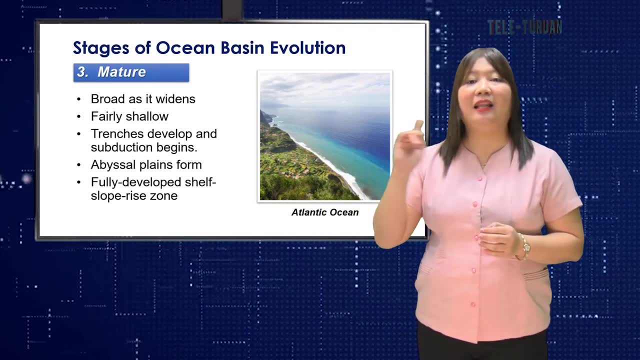 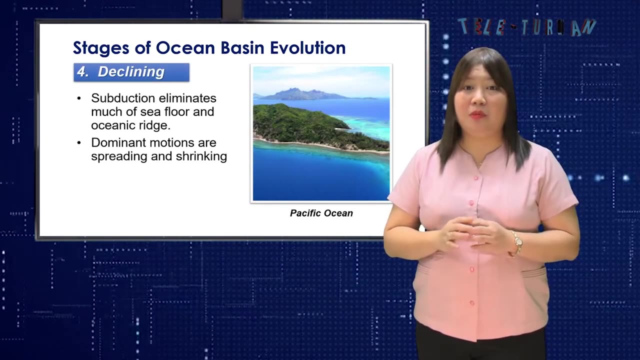 continental sharp slope rise zone becomes fully developed. The continental margins are more or less parallel to the central spreading ridge. as in the Atlantic Ocean, Stage 4 is a declining ocean basin when subduction eliminates much of seafloor and oceanic rids. 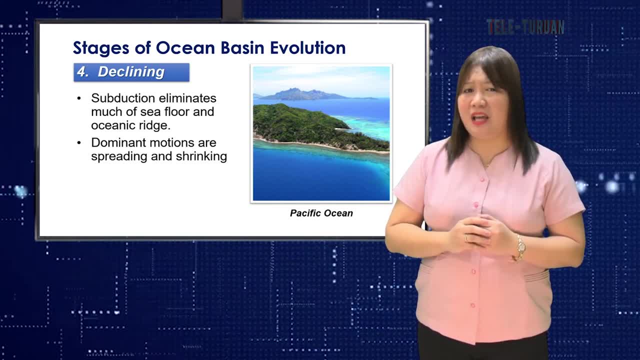 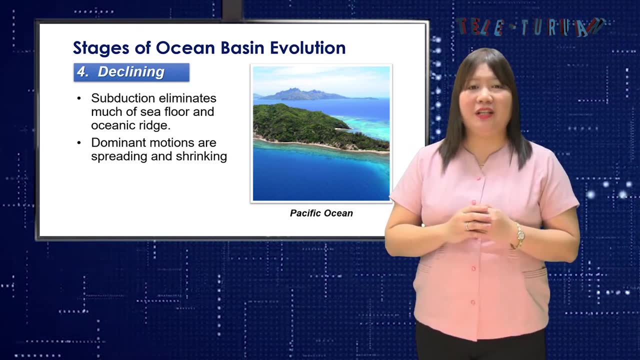 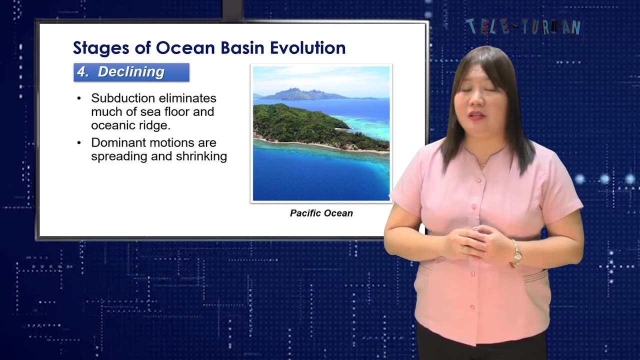 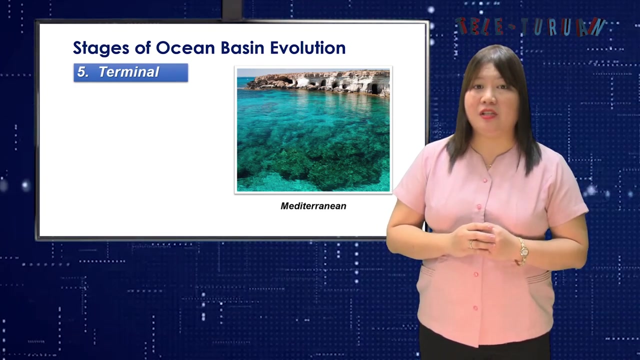 The reason for the formation of new destructive margins probably lies in changing circumstances in another part of the globe, such as continental collision or the initiation of new continental rifting. Dominant motions are spreading and shrinking. an example is the Pacific Ocean. The Mediterranean is an ocean in the final stages of its life, in Stage 5, with the African. 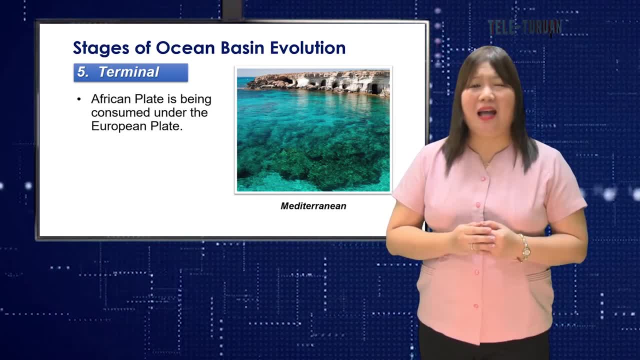 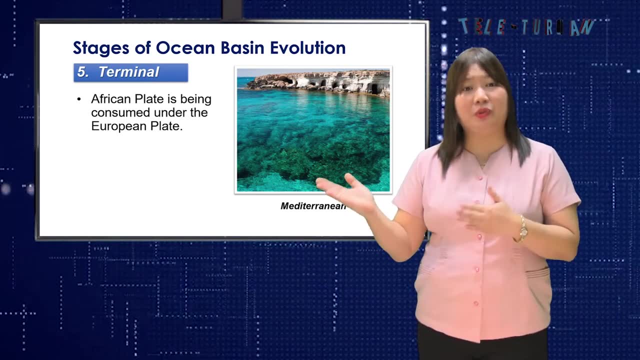 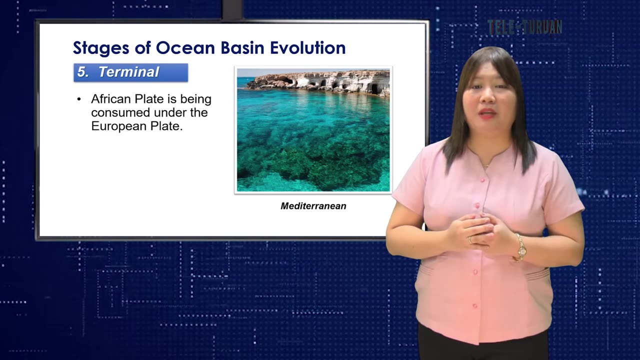 Plate being consumed under the European Plate and thus the world system of plate stages, so as to help the northward movement of Africa relative to Europe. The continental blacks of Europe and Africa will eventually collide and new mountain ranges will form in Stage 6..